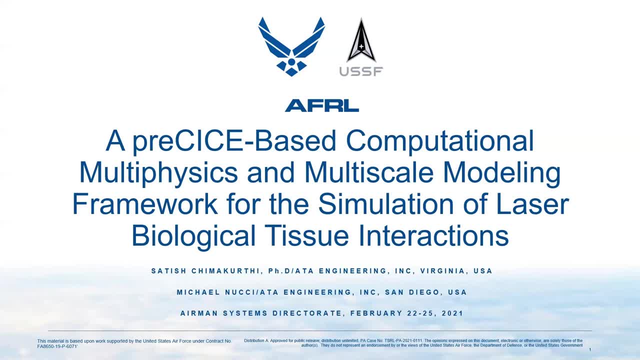 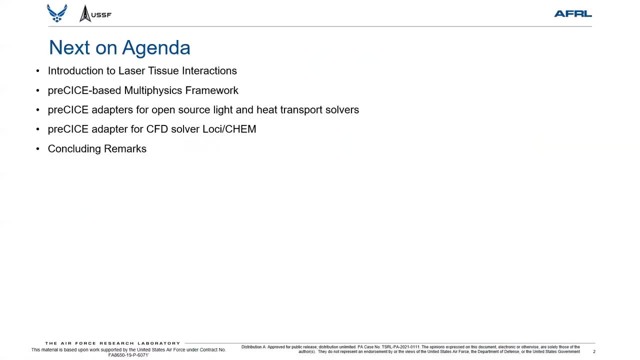 point of contact, Dr Andrew Womby, who works out of the Air Force Lab in Fort Sam Houston, Texas. This is a brief outline of our talk today. I will first provide a very quick introduction to laser tissue interactions and then provide an overview of the pre-size-based multi-physics. 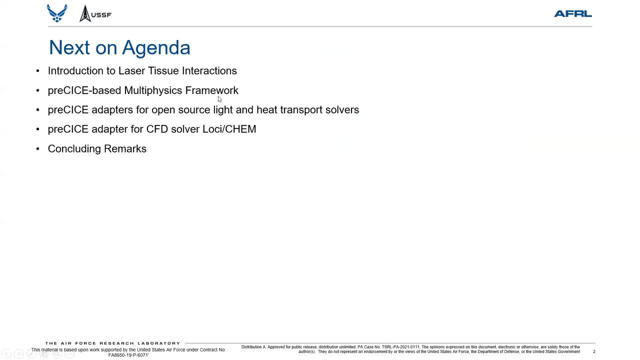 framework that we prototyped for this project. After that, Mike and I will briefly discuss pre-size adapters for a light transport and a light transport. for a light transport, The project will also focus on mass transfer, heat transport and a computational fluid. 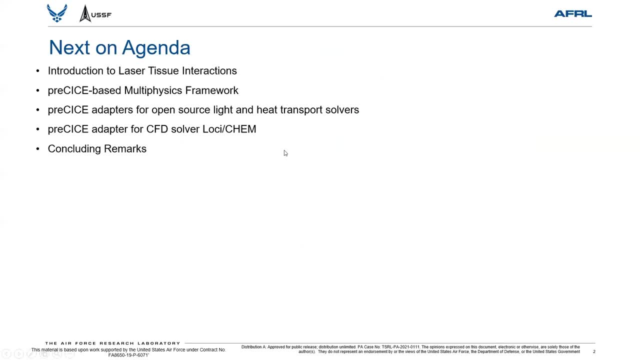 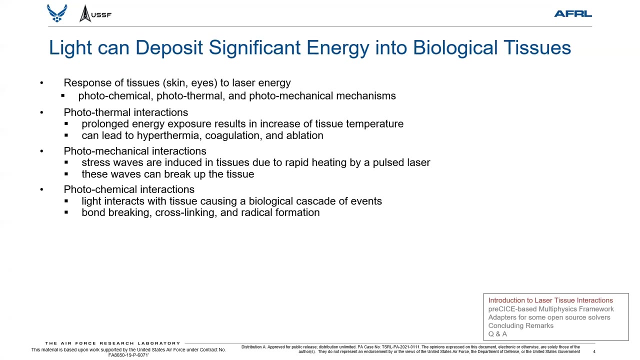 dynamics solver called LociChem, all of which were developed as part of this project. We will then present some preliminary results from our verification study and finally make some concluding remarks before opening up the floor for Q&A. Moving on Basically, after energy deposition, lasers can interact with biological tissues. 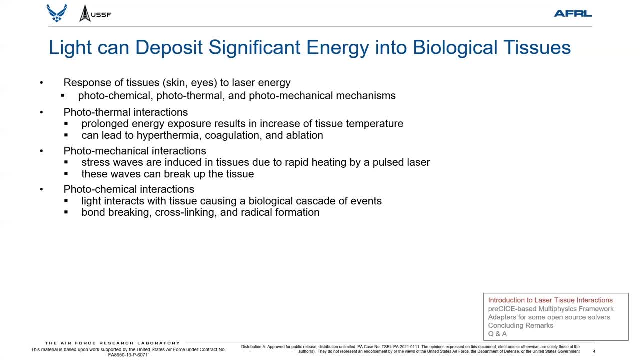 in many ways, And the interactions generally involve physical mechanisms that can be based on photochemical, photothermal and photomechanical effects, Which means that the laser can interact with the physical mechanisms of the ότιomim, Krundstrom and Newtonian molecules And then 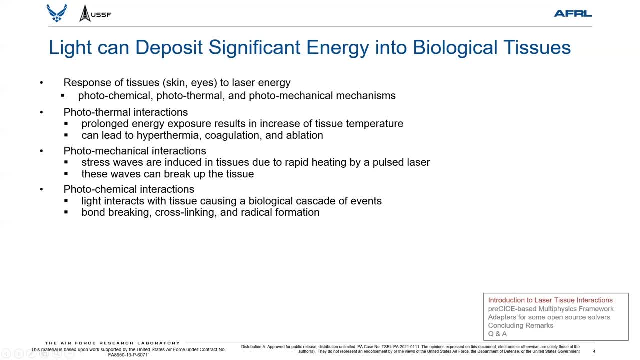 the laser can interact with the biocompatible elements of the LpC process. These interactions are effects and these mechanisms involve some basic physical phenomena such as light transport, thermal transport, hydrodynamics and stress wave propagation In photothermal interactions. 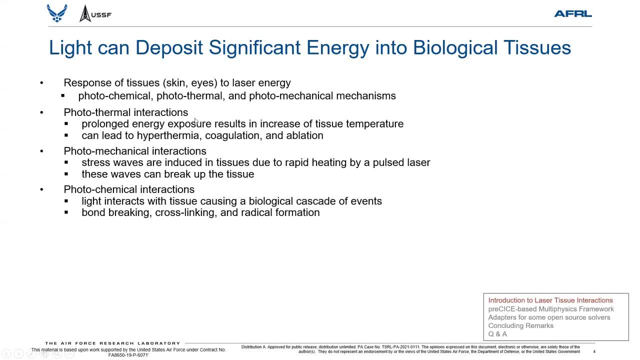 temperature is the governing parameter. Depending upon the temperature rise and duration of exposure, different tissue effects, such as hypothermia, coagulation and ablation, occur In photomechanical interactions. stress waves are induced in tissues due to rapid laser heating and under certain conditions, the waves can even fragment, that is, break the tissue. 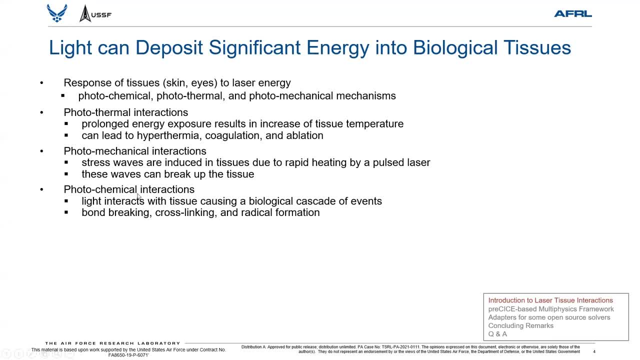 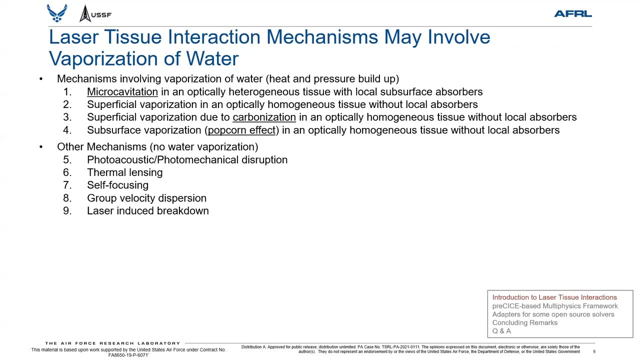 out. Finally, in the photochemical case, light can interact with tissues and cause a cascade of biological events, such as bond breaking, cross-linking and radical formation, to occur. There are many laser tissue interaction mechanisms and I've listed some here. 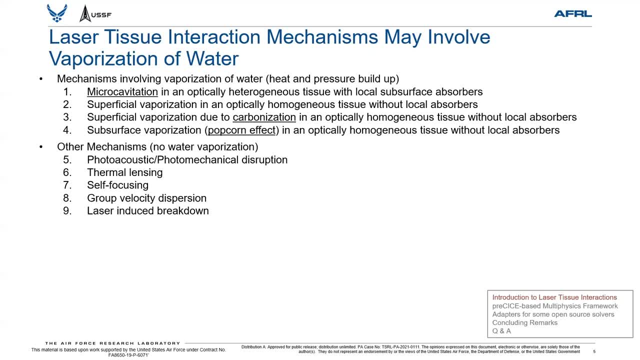 They're all broadly classified into two categories: Those that involve vaporization of water and those that don't. I won't go through this in detail, but I just wanted to point out that microcavitation, carbonization and popcorn effect that you frequently encounter in literature. 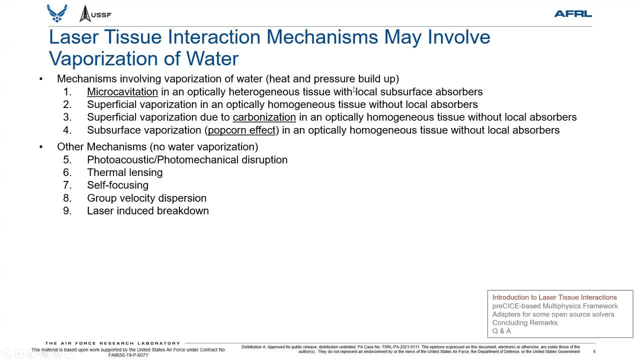 involve vaporization of water and subsequent heat and pressure buildup within the tissue And photo-ecosystem disruption. thermal lensing, self-focusing are some examples of mechanisms that do not necessarily involve vaporization of water And, lastly, there are some mechanisms such as self-focusing, laser-induced break. 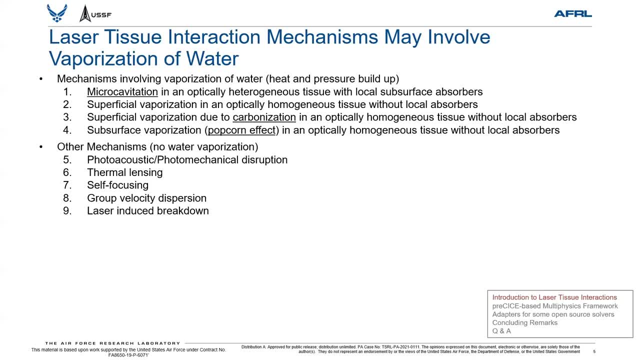 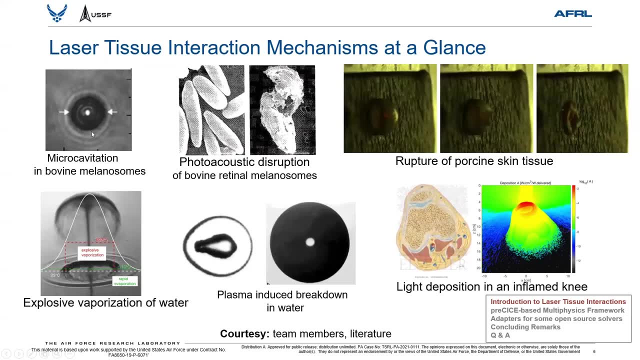 down that involve nonlinear effects. Here are some original photographs from experiments showing various laser tissue interaction mechanisms in action. First, on the left-hand side top, we have microcavitation in melanosomes that deals with vapor bubble formation and expansion. in some 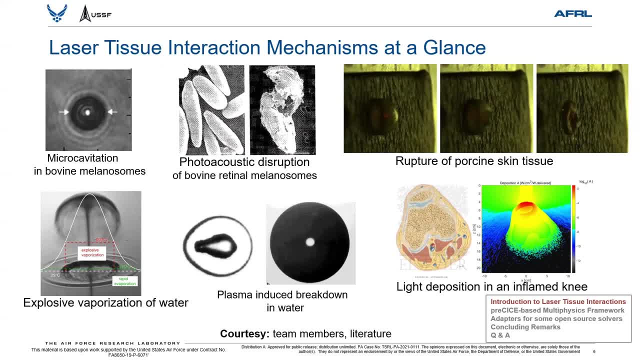 tissues. As you may be aware, melanosomes are pigmented granules that are found in the retinal pigment epithelial RPE cells in the eye and in keratinocytes of pigmented skin. The second one at the top is a picture showing photo-ecosystem disruption and bovine retinal 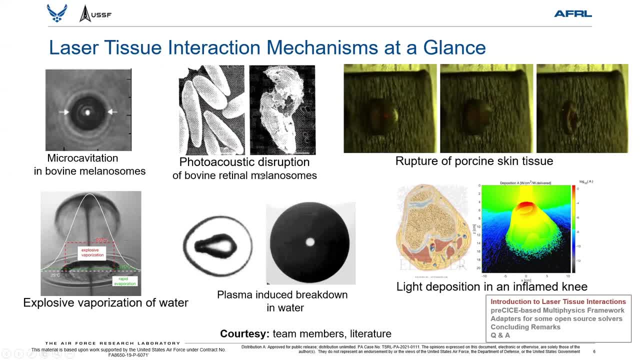 melanosomes, wherein the damage occurs due to stress waves and wave reflections in material interfaces. And then the picture on the right-hand side top corresponds to rupture of skin tissue due to rapid vaporization of water, And there are many other mechanisms such as explosive vaporization. 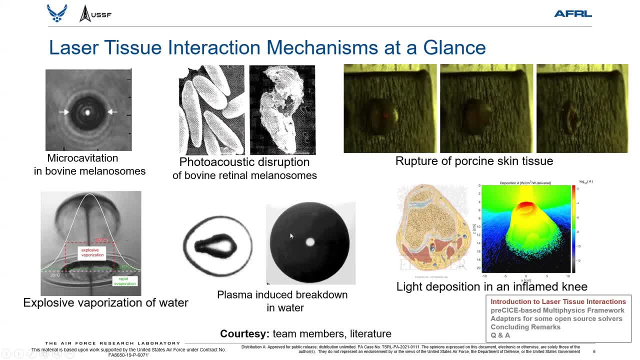 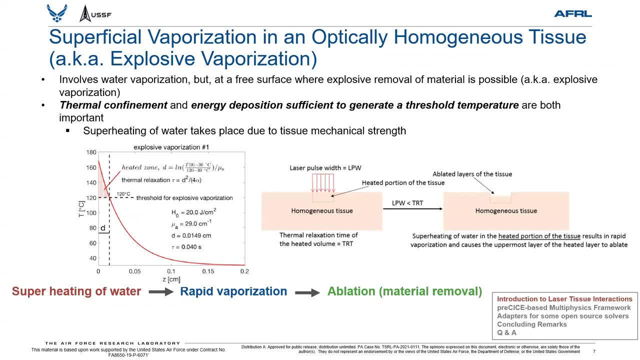 plasma-induced breakdown that you see here, and all of which are some examples of laser tissue interaction mechanisms. In the interest of time, we'll just go through the explosive vaporization mechanism in some detail in the next slide. Explosive vaporization involves superheating of water at a free surface. 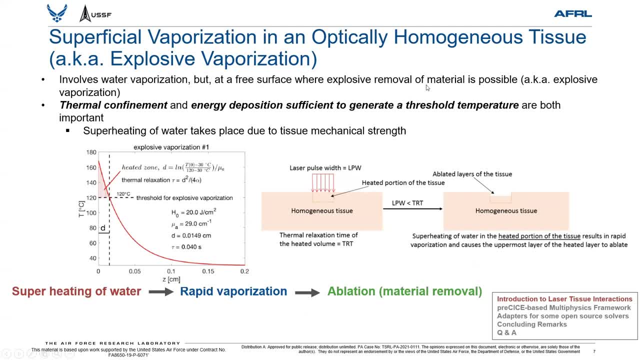 and rapid vaporization and subsequent material removal in a tissue that is basically optically homogeneous, And in this mechanism, both thermal confinement as well as energy deposition that is sufficient to generate a threshold temperature are both important. Basically, thermal confinement happens when your laser pulse duration is. 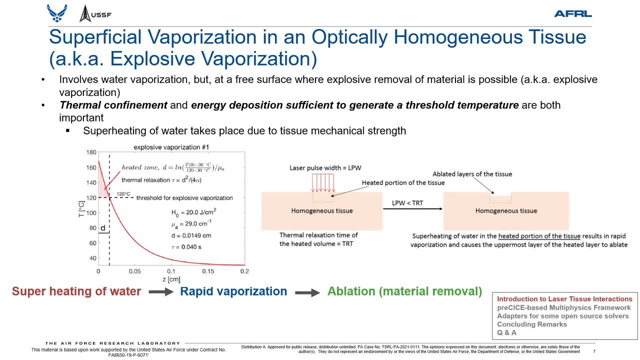 shorter than the thermal relaxation time, which is the time taken for the absorbed laser energy to dissipate away by thermal conduction. The picture you see on the left-hand side bottom corresponds to a plot of tissue coordinate on the x-axis and temperature on the y-axis. 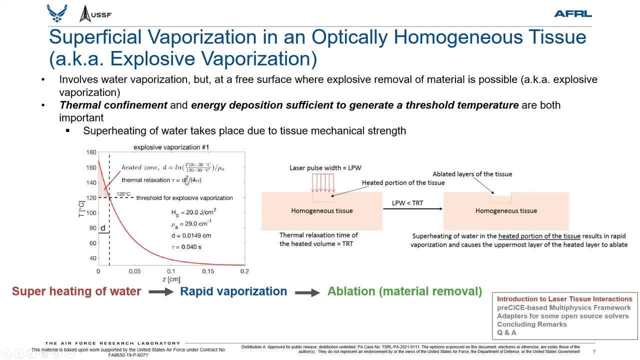 Coordinate z, equal to zero, corresponds to the tissue surface. What this plot says is that once the temperature of the heat is reduced, the temperature of the temperature of the thermal relaxation time is reduced. In this case, the heated zone near the free surface is above a. 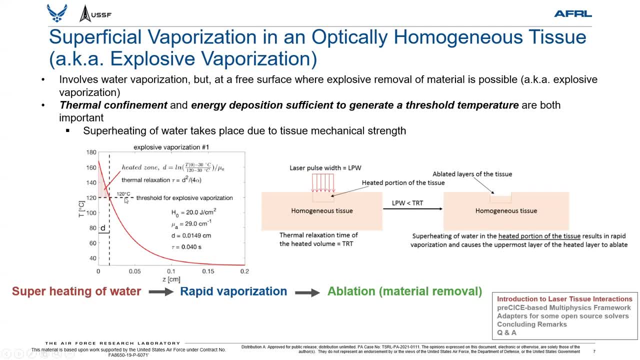 threshold- In this case it is 120 degrees Celsius- Explosion occurs and material is removed, and that is shown somewhat crudely in the second picture here, where you see a block of homogeneous tissue that's being irradiated with a pulsed laser over the LPW. that is less than the thermal relaxation time denoted as TRT. 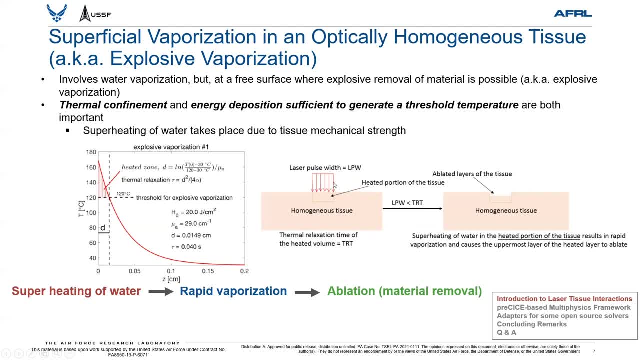 Basically, what's happening here is that superheating of water takes place, leading to rapid vaporization. This causes the uppermost layers of the heated portion of the tissue to ablate. I'd like to emphasize that the threshold temperature we are discussing here 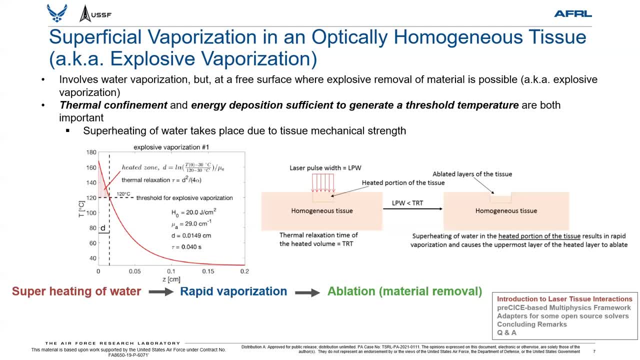 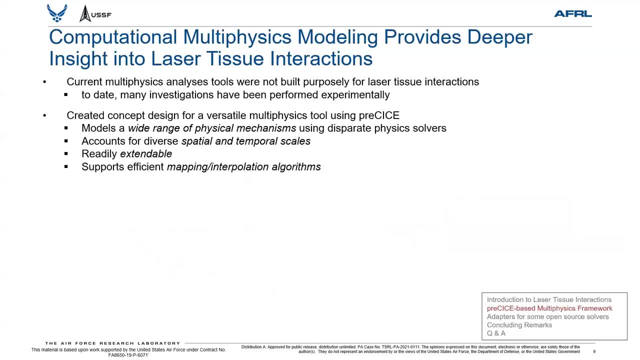 is highly variable and is obviously dependent upon the mechanical strength of the tissue Moving on. so, as you can imagine, laser tissue interaction modeling requires a wide range of physics capabilities, including light transport, heat transport, tissue damage, fluid dynamics, mechanical damage and molecular dynamics, and you want a versatile. 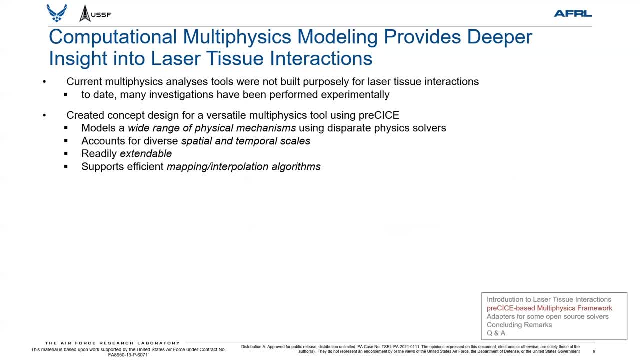 multi-physics tool that incorporates all of this physics. However, the tools that are currently available in literature were not built especially for the purpose of laser tissue interactions, and also many investigations in this area so far have been performed experimentally. Keeping this in mind, we developed and prototyped a versatile multi-physics framework using pre-size. 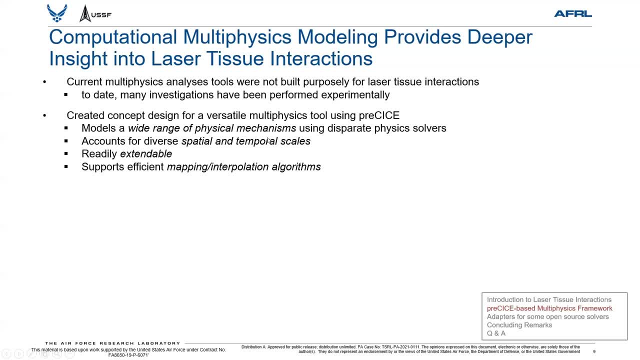 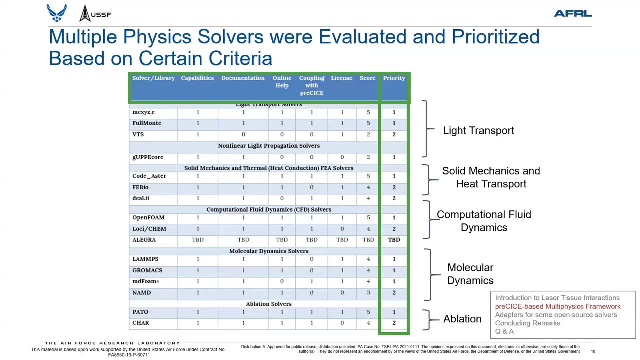 to be able to model a wide range of physics, to account for diverse scales and also to create an extensible software framework. In order to accomplish this, a number of single physics solvers were chosen and some adapters were written to couple them all with pieces. So, as you can see in this table, the project team has evaluated. 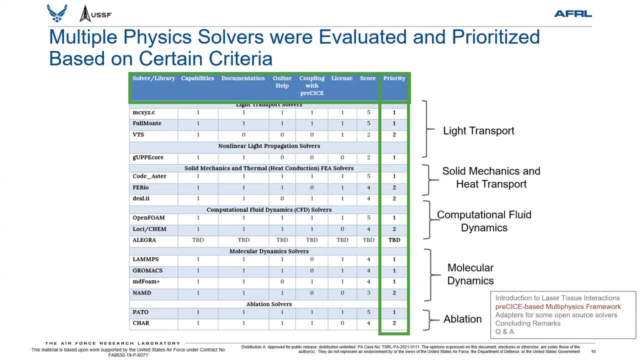 a number of open source physics solvers and prioritized them based on some criteria, including capabilities, availability of good quality documentation, online health, whether or not the solver is already coupled with pre-size licensing. flexibility. and final scores are shown in this table for each of the solvers in the light, transport, solid mechanics and heat. 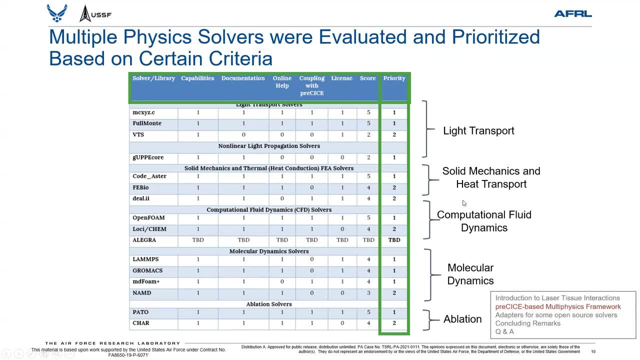 transport, CFD, molecular dynamics and ablation categories. So, for example, for light transport, we ended up choosing two open source solvers called MCXYZC and FullMonte as the top priority ones. Similarly, we chose a non-linear optics solver called GF-Core, and for CFD, 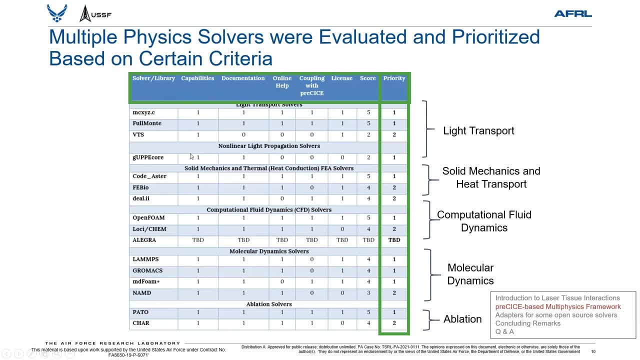 we chose OpenFoam and LociCAM. Our idea has been to first focus on the top priority solvers in each of these categories, but eventually bring the lower priority ones as well into the mix. Of course, as you can imagine, if new information comes in, the solvers may need to be reprioritized. 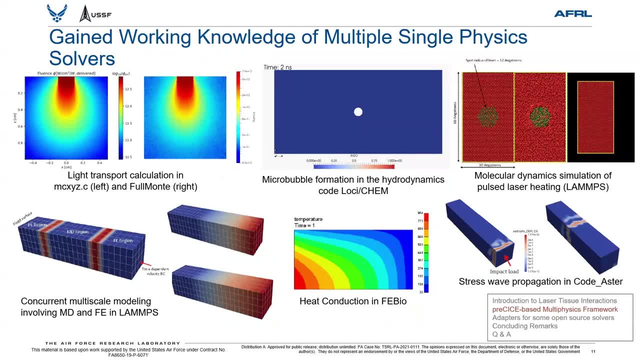 And in order to come up with the priority ratings for the solvers, we gained some working knowledge of each of them by setting up and running some demonstration-level problems. This slide and the next one are snapshots of some of the solvers that we've been working on for a long time. We've also 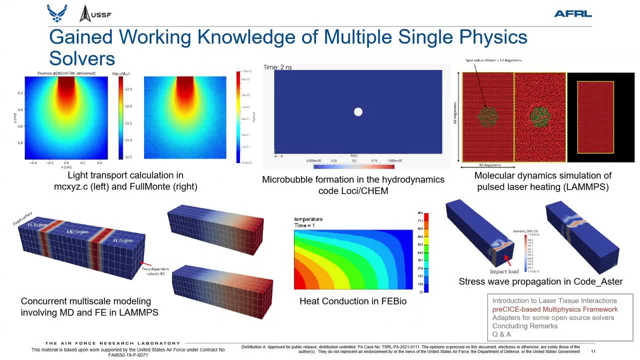 done some results from simulations that I wanted to highlight. You know I recognize this slide is a bit busy, but I'll quickly walk you through it. The picture on the left-hand side top corresponds to light transport results obtained from a tissue sample modeled MCXYZC. on the left and compared to: 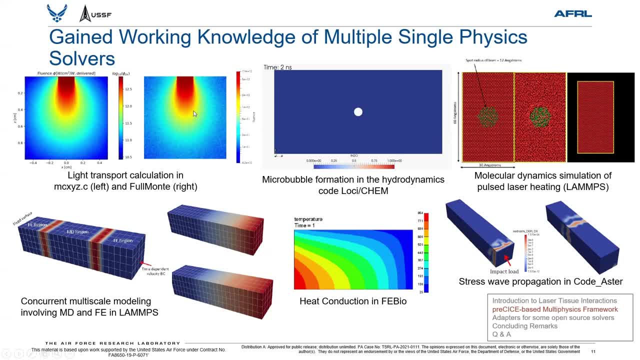 those of a FullMonte simulation on the right, and both have agreed with each other. The animation that you see here on the top at the center shows the evolution of a vapour bubble around a laser-heated wall. This was modeled in low-psych chem. 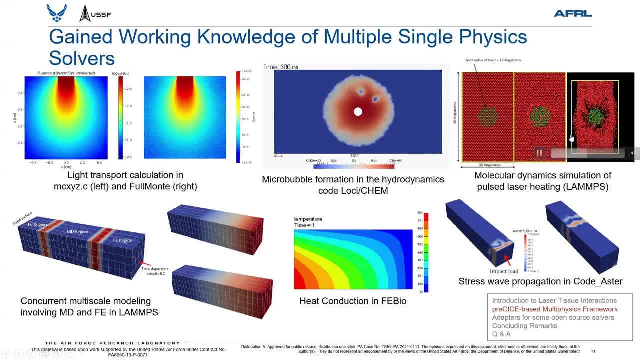 And the animation here corresponds to a very simple and rudimentary molecular dynamics simulation of pulsed laser heating that was set up in lamps. In this manner we gain working knowledge of other solvers as well, including the biomechanics FE solver, FEbio and the open source nonlinear FE solver. 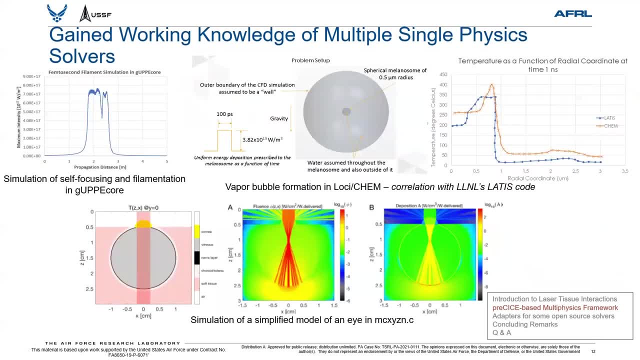 Codaster. Along the same lines, we also gain working knowledge of a nonlinear optics solver called GF-Core, which is being developed at the University of Arizona by Professor Miroslav Kolesnik. I won't go into these in any detail. 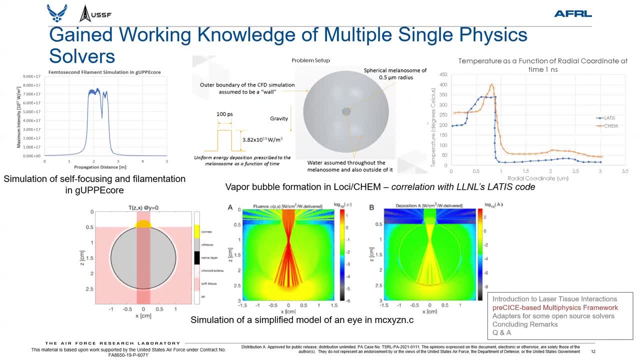 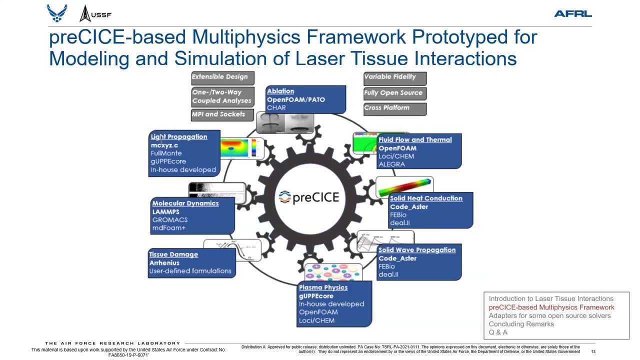 but I hope you get the idea behind this exercise. Overall, the multi-physics framework created with Precise involves fully open source cores and is able to simulate a variety of laser tissue interaction mechanisms. Again, as I mentioned, this framework supports multi-physics coupled workflows involving 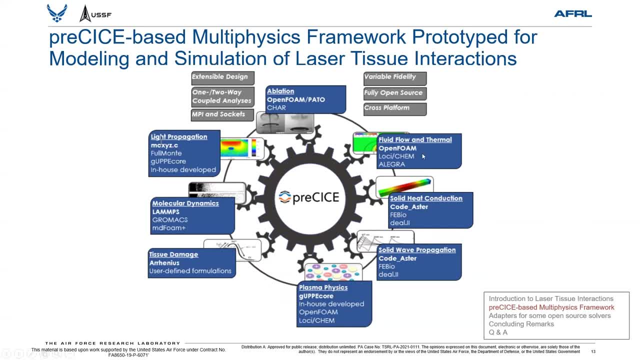 a variety of physics involving light transport, fluid flow and thermal heat conduction and the solid wave propagation, plasma physics and molecular dynamics as well, And I don't have to tell this audience about all the different coupling schemes that Precise supports. 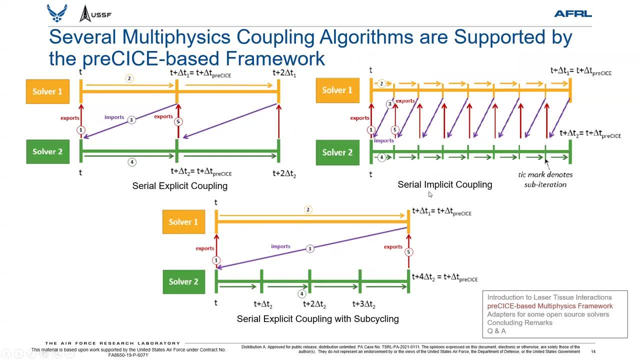 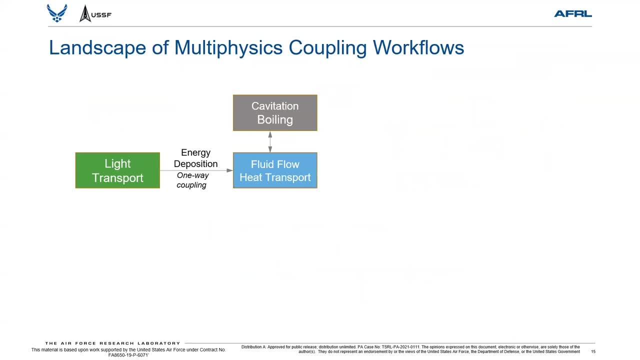 including, and not limited to, serial explicit, serial implicit and serial explicit with subcycling. On the whole, there is a landscape of multi-physics coupling workflows that we can talk about in the context of laser tissue interactions. If your interest is in, let's say. 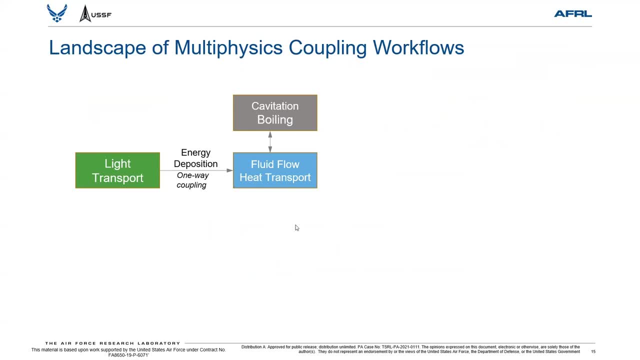 simulating microcavitation without damage. you can have a one-way coupling between a light transport core and a fluid flow and heat transfer core. If you then come and say that you're interested in having dynamic optical properties, you end up with potentially a three-way coupling involving 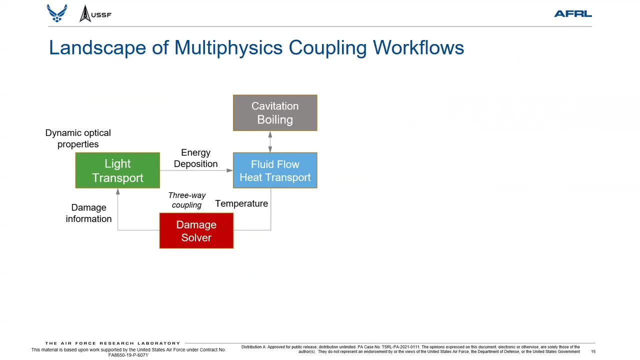 light transport, fluid flow and the damage solver, And then you can introduce a solid, deformable component in the tissue and account for fluid-solid interaction. Then you can say that your solid not only deforms, but also conducts heat, And so you add a one-way coupling. 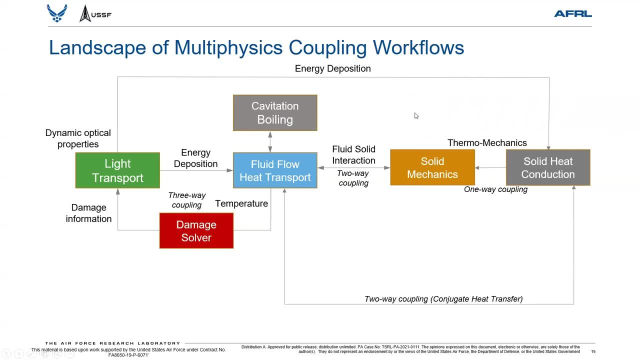 You can have a thermomechanics coupling here And you can have conjugate heat transfer with the fluid dynamic thermal properties and solid mechanical damage and ablation. You can also have multi-scale coupling, molecular dynamics. And then, lastly, you can replace the light transfer block here. 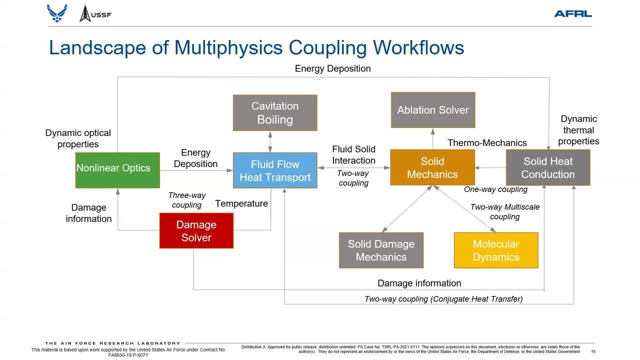 with nonlinear optics to account for nonlinear effects. I know that this is a very busy slide, But basically the point of this is to show that, depending upon the type of the material, the amount of energy that is used to simulate the pre-size-based multi-physics coupling workflow, 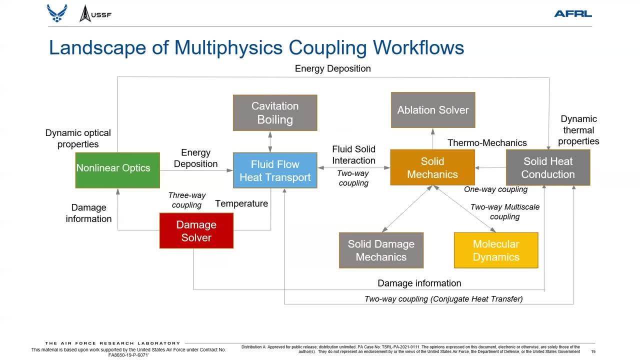 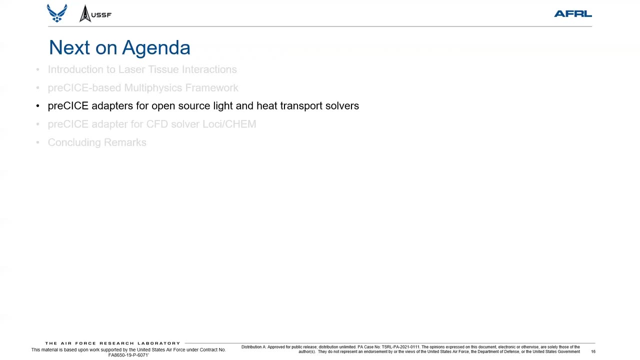 can grow or shrink And, obviously, simulation of a landscape such as this one must therefore be done very systematically, incrementally and iteratively, while doing B and V at each stage. So, moving on, in order to demonstrate multi-physics couplings for pre-size using a light transport and a heat. 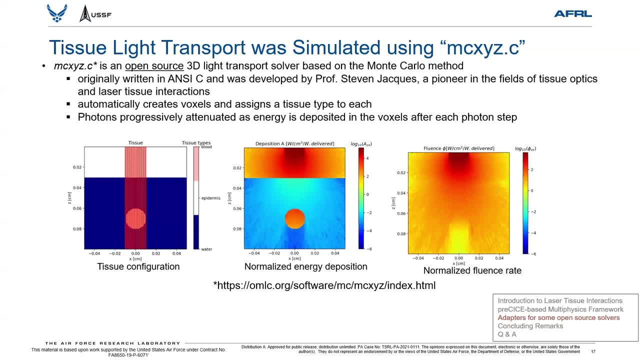 transport solver, we created a couple of pre-size adapters that we will talk about next. So the light transport solver that we considered is mcxyzc. As I mentioned, it's an open-source solver based on the Monte Carlo method and was written by Professor Steven Jacks, who is a partner of ATA Engineering. 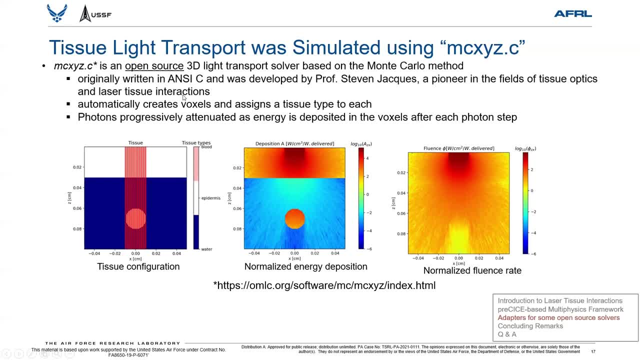 on this project and is one of the pioneers in the fields of tissue optics and laser tissue interactions. Basically, the code creates a 3D grid of voxels and assigns a tissue type to each of them, And photons are launched from a given location on the surface of the tissue. 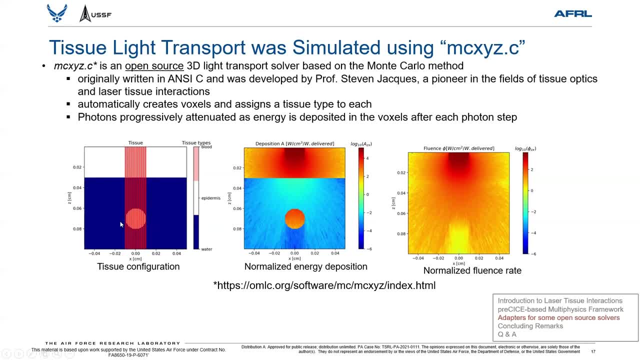 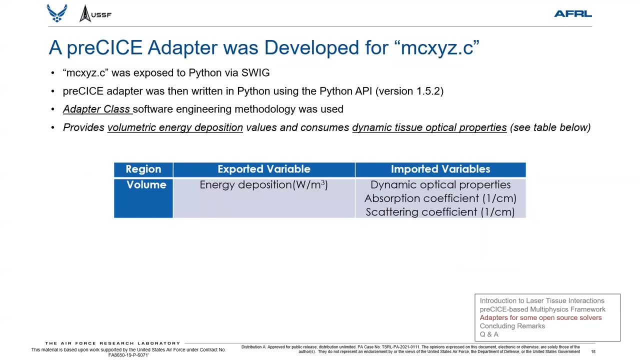 and are then tracked to the tissue as they get absorbed and scattered and eventually getting attenuated. The normalized energy deposition, and normalized through and straight, are coupled with output quantities from the solver And the pictures here correspond to the same. So originally mcxyzc was written in NCC and given our interest to develop. 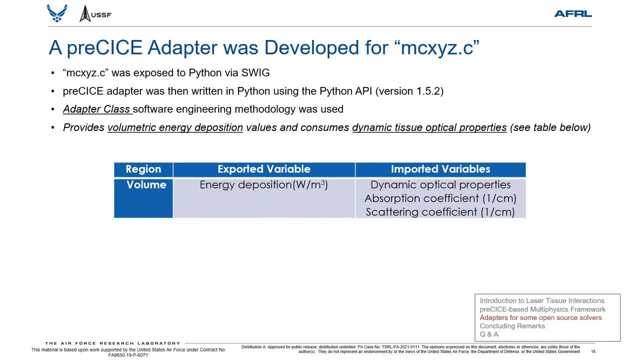 the adapters in Python. we wrapped the SQL up using SWIG and then used the adapter class methodology to create the pre-size adapter. Now, as seen in this table, the adapter is able to export volumetric energy deposition values and import optical properties, including the tissue. 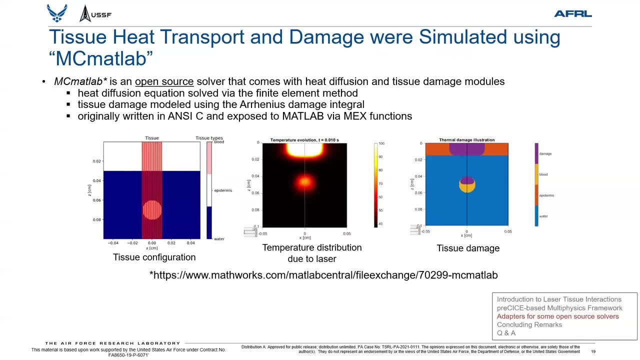 absorption and scattering coefficients. Given our interest to demonstrate the coupling of the light solver, mcxyzc, with the tissue heat transport and damage solver, we picked up an existing open-source solver called MCMETLAB. Basically, this code solves the heat diffusion equation, coupled with the 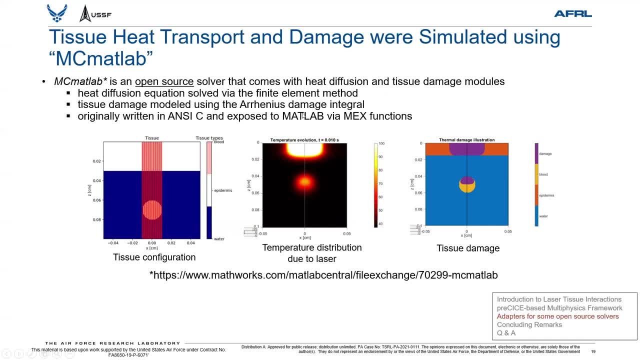 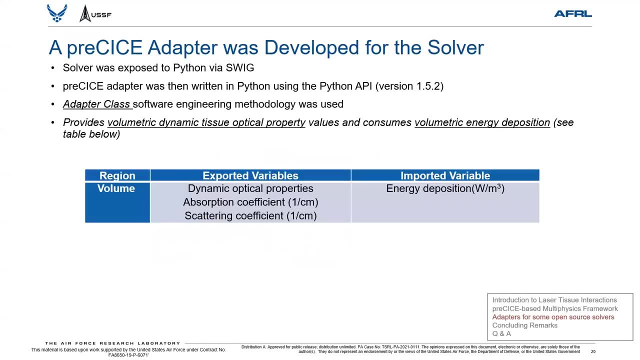 Arrhenius damage integral to moderate heat diffusion and tissue damage respectively. The core solver is written in C But exposed to MATLAB-IMX functions. Again, given our interest in developing the adapter in Python, we wrapped the C code up as usual via SWIG, and then a pre-size adapter was created. 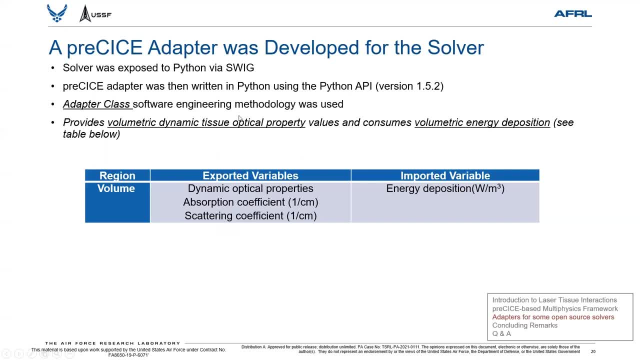 using the adapter class software engineering methodology, As shown in the table here. this adapter exports optical properties, including absorption coefficient and the scattering coefficient, and imports energy deposition. So basically, this is doing exactly the opposite of what the adapter from mcxyzc is said to do. 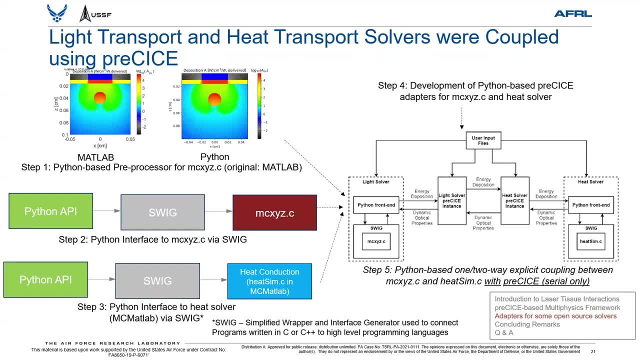 With the Python-based adapters for mcxyzc and the heat solver named heatsimc, here both in place. they were coupled using pre-size. Currently, for this coupling, only the serial explicit scheme is supported. The pictures here simply show the incremental steps we took to develop. 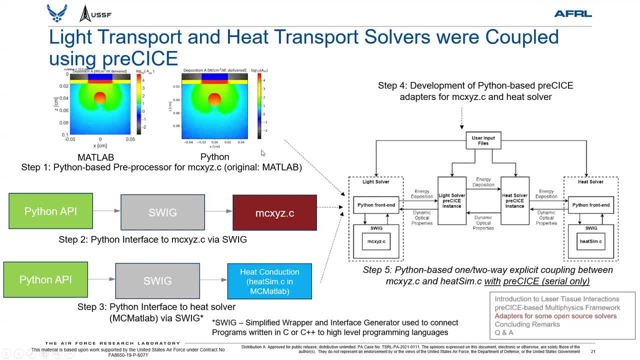 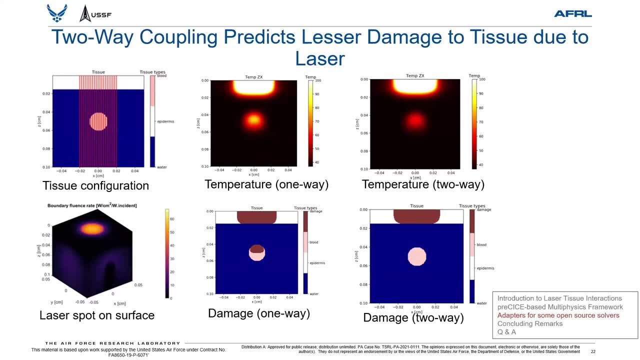 the coupled code, and I'm not going through this in any detail. We tested the one-way and two-way coupling capabilities using a demonstration case that we found in the literature. What you're looking at here on the top left is a tissue configuration that is composed of a layer of epidermis that you see in white at the top. 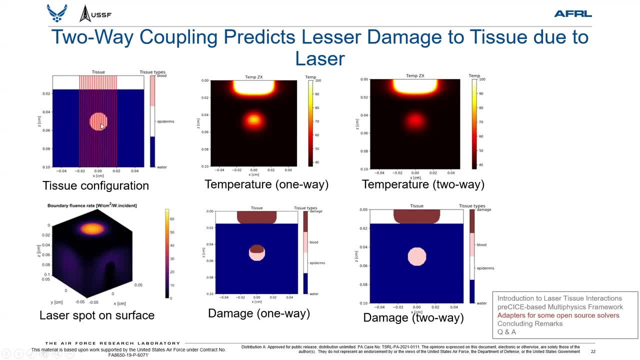 water at the bottom in blue, and a blood vessel at the center in red. This geometry is in 3D, but what you're seeing here is just a slice-up. The picture on the bottom left corresponds to the location of the laser spot of 0.02 centimeter radius on the surface. 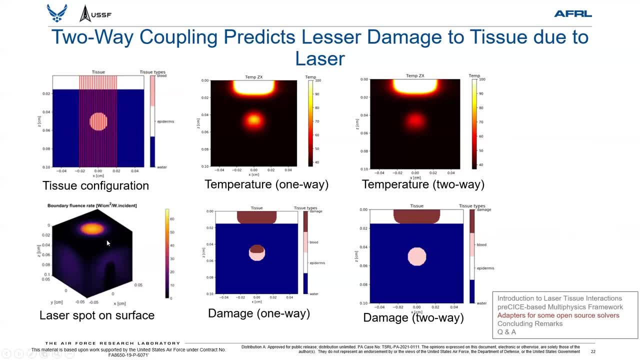 It's a 5-watt laser with a wavelength of 500 nanometers that is irradiating this tissue for 0.01 seconds. The two pictures in the second column here correspond to the temperature distribution and tissue damage computed with the coupled code with one-way. 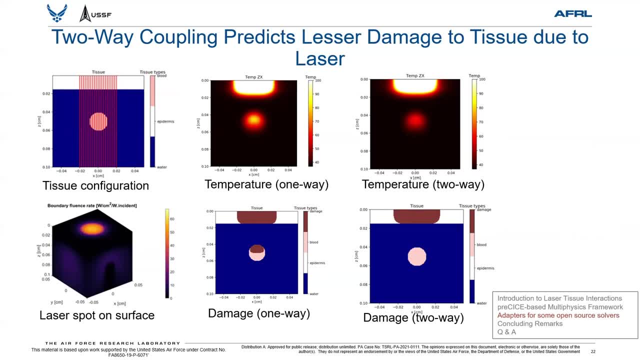 coupling, that is the one without dynamic optical properties. When you compare the results in this one-way case with those of the two-way that includes dynamic optical properties, you'll see here that in the two-way case the magnitudes of the temperature are lower. and also if you look at the 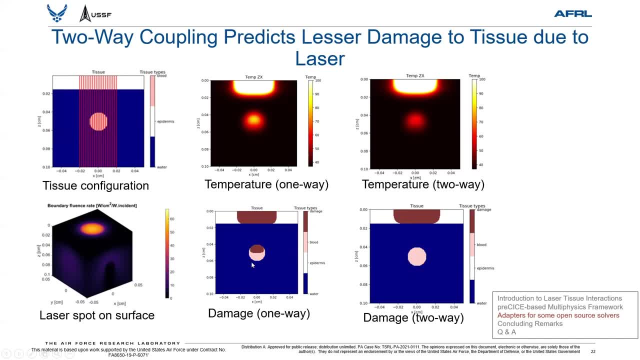 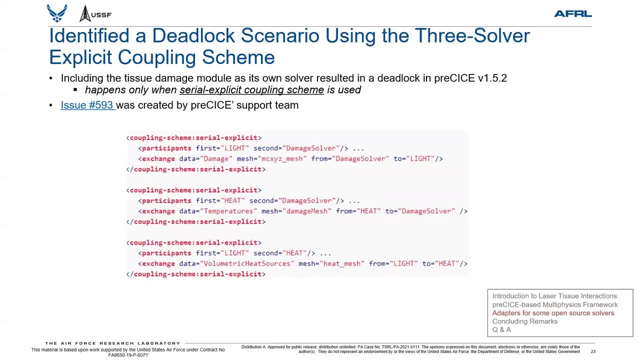 blood vessel. you do not see damage that you otherwise see in the two-way case. The results that you just saw are from a coupled code involving only two solvers: light transport and another solver that computes both heat diffusion as well as tissue damage. 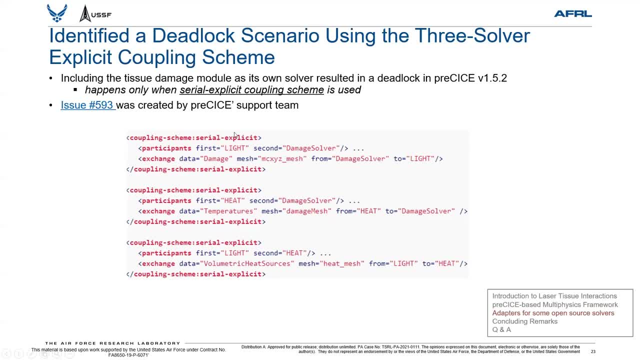 During the course of this project, we attempted to try the serial explicit coupling scheme using three solvers, including light transport, heat transport and then an independent tissue damage solver. However, we reached a deadlock with the setup. We got in touch with Precise Support and we were advised to use a fully 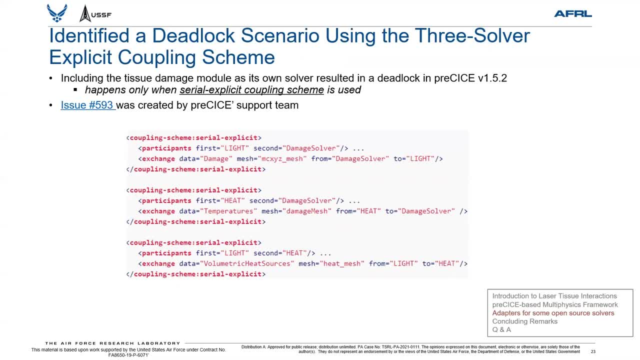 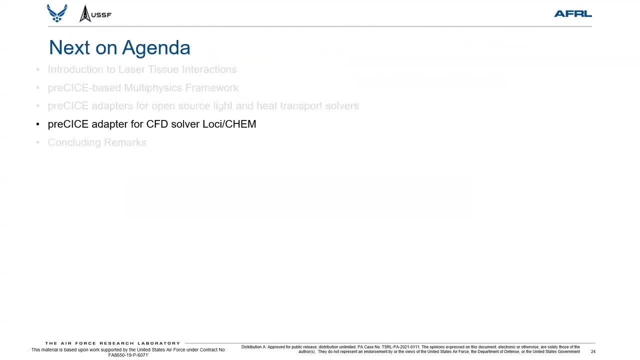 implicit coupling scheme until this is resolved. An issue was created by the support team and I just thought I should mention this, So at this point I would like to hand this over to my colleague, Mike Nochi, who's going to talk about the Precise Adapter that we created for a CFD solver. 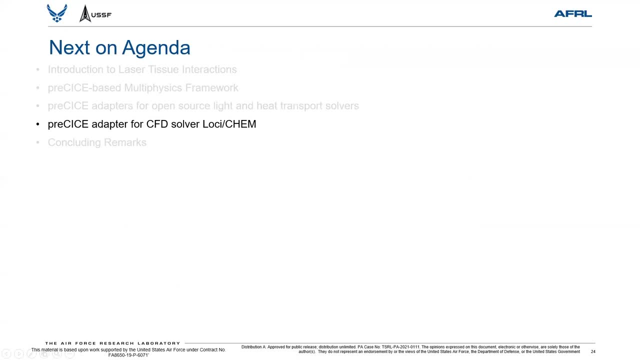 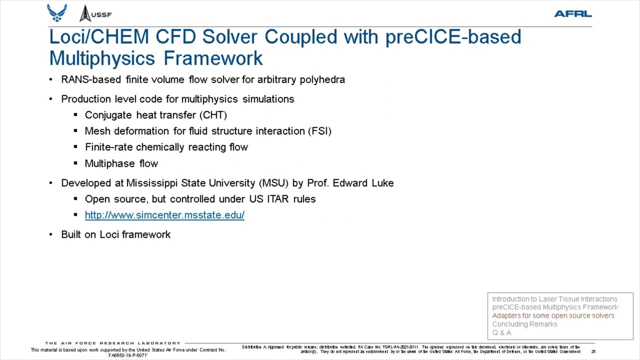 called LociCAM. Mike, it's all yours now. Thanks, Satish, I'll take the next couple of minutes. I'll take the next couple of minutes to talk about the Precise Adapter for LociCAM. LociCAM is a RANS-based finite volume flow solver for arbitrary polyhedra. 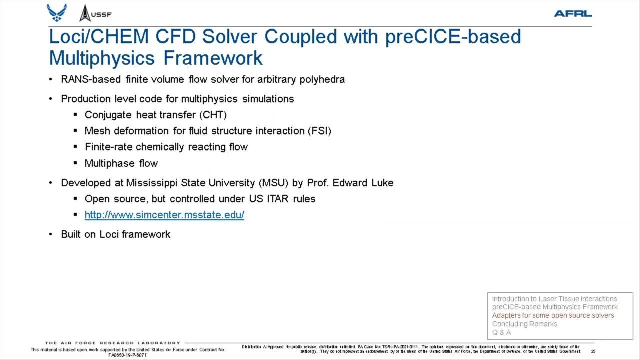 It's the production code at NASA Marshall and widely used at many other NASA centers. It has some key features making it ideally suited for multi-physics simulations. For example, it has a conjugate heat transfer model, a robust mesh deformation algorithm for fluid-structure interaction, a finite-rate chemical reaction. 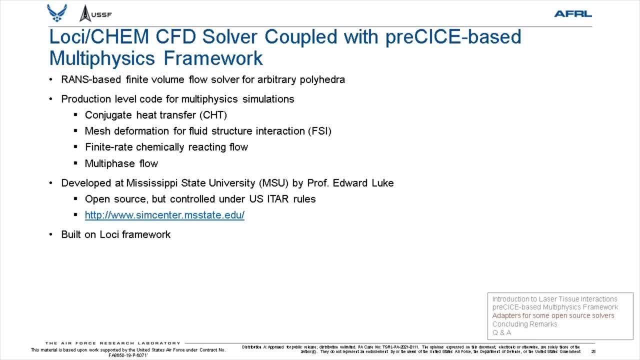 flow model and a multi-phase flow model, LociCAM, was developed at Mississippi State University by Professor Ed Luke. It is open source but controlled under US ITAR rules. It is distributed by Mississippi State University as well, and a copy can be requested from. 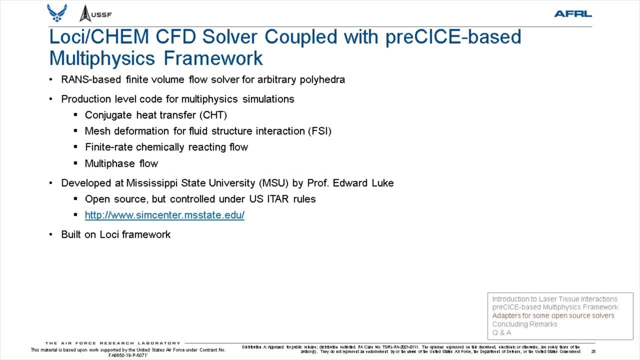 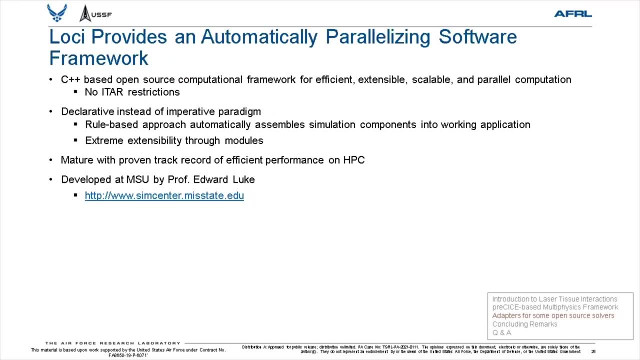 the link shown, CHEM is the application name and it is built on the Loci framework, hence the name LociCAM. Loci is a C++-based open source computational framework. It has no ITAR restrictions and is completely open source. 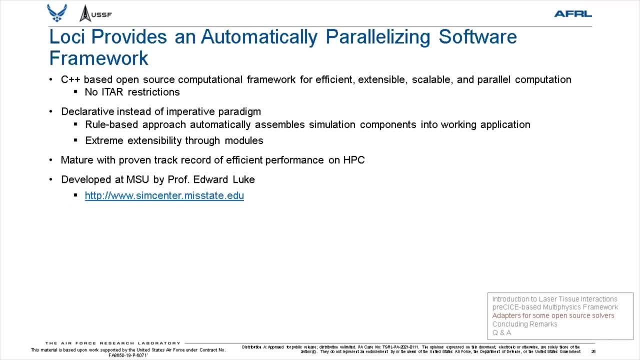 It allows for efficient, extensible, scalable and parallel computation. Loci uses a declarative instead of imperative programming paradigm. It uses a rule-based approach to automatically assemble simulation components into a working application. In Loci parlance, a rule can be thought of as a computational 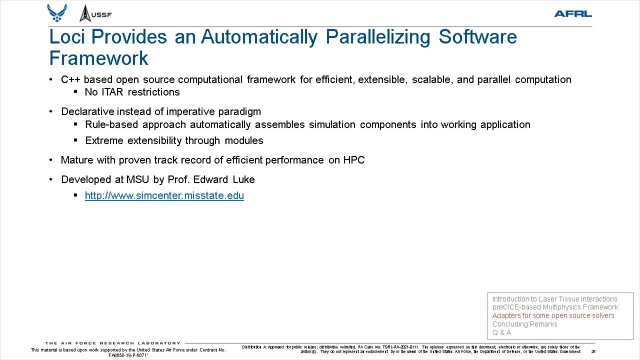 unit that has inputs and outputs Within the source code. the rules can appear in any order and at runtime Loci deduces the execution order based on their inputs and outputs to the respective rules. Loci allows for extreme extensibility through its modules, which I'll discuss in the coming. 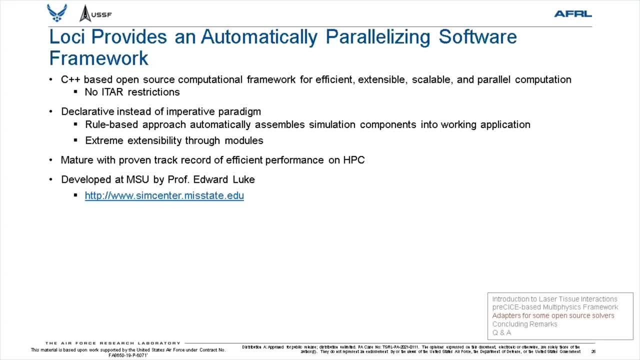 slides. It has a mature, proven track record of efficient performance on H3CAM and H3CAM. It has a high level of performance. It is also developed at Mississippi State University by Professor Ed Luke, and a copy of Loci can be requested from the links shown. 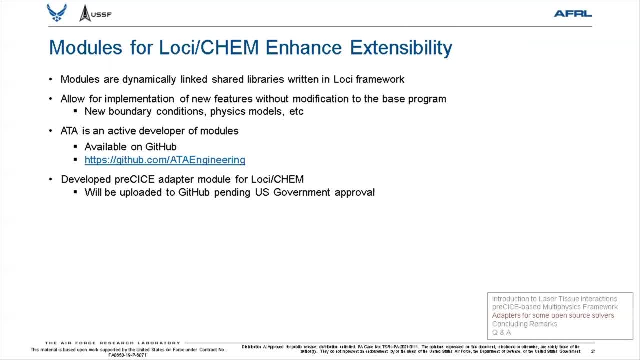 Modules greatly enhance the extensibility of LociCAM. Modules themselves are dynamically linked, shared libraries that are written in the Loci framework. They allow for the implementation of new features without any modification to the base program. Modules can be used to add new boundary conditions, physics models, such as turbulence models. 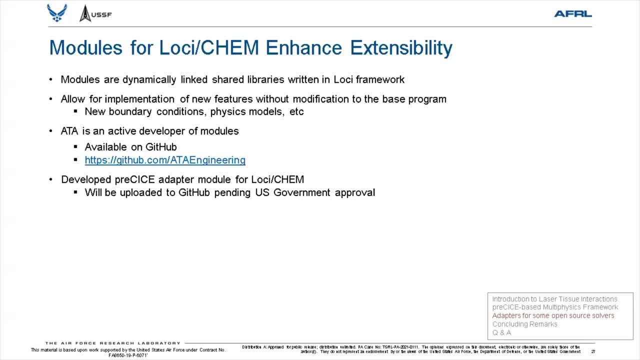 coupled to other codes or even enable the output of new variables At ATA. we're active developers of modules for LociCAM. Many of these modules are available on our GitHub page. The link is shown there. This precise adapter module that we have developed for LociCAM: we also plan to upload it to. 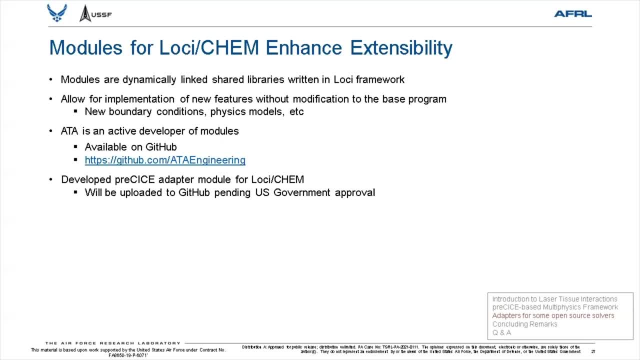 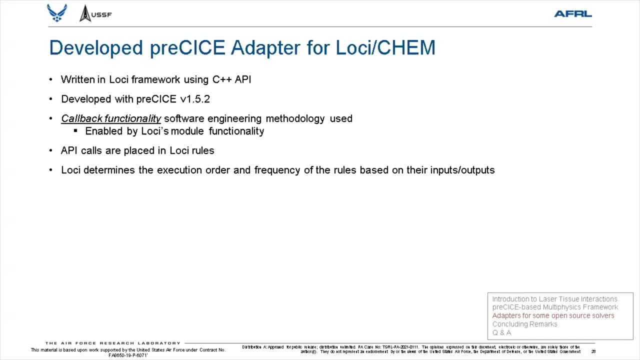 our GitHub page, pending approval from our US government sponsors. The module developed for LociCAM for the Precise adapter was written in the Loci framework using Precise's C++ API. It was developed with Precise version 1.5.2, as that was the latest version at the time. 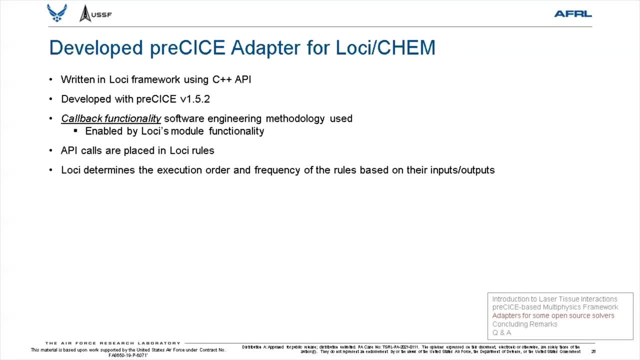 of development. It uses the callback functionality software engineering methodology. This means that the base code does not have to be modified and all of the logic for the module and the Precise API calls- all of that is self-contained within the module And this is enabled by Loci's module functionality. 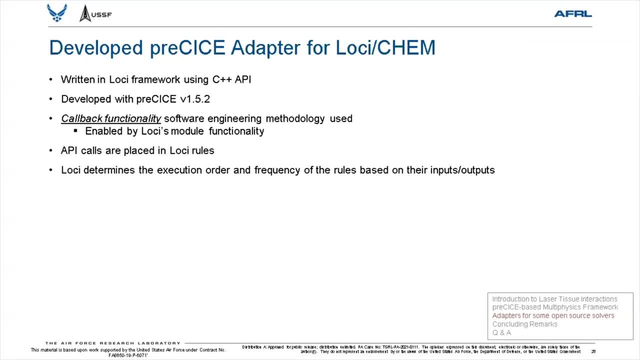 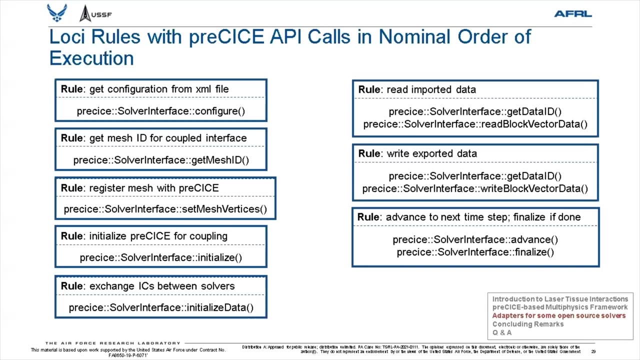 The Precise API calls themselves are placed in Loci rules and then Loci will determine the execution order And the frequency of those rules based on their inputs and outputs. This shows an abstract representation of the rules that are present in the module. 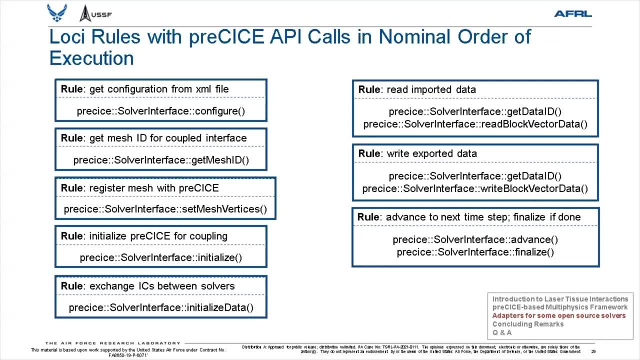 Remember that in the source code the rules can appear in any order, but on this slide they're nominally in the order of execution: First the left column top down and then to the right column top down. So each rule will have a purpose. 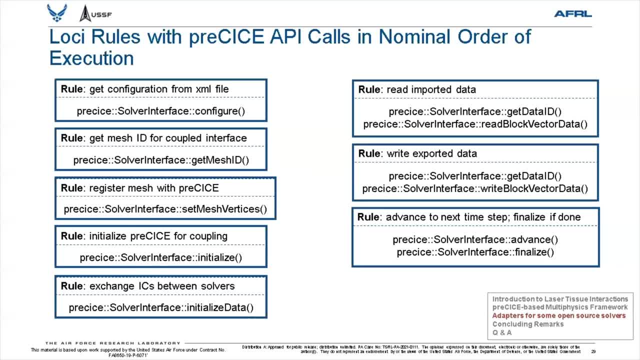 For example the first rule. the purpose is to get the configuration from the XML file. So in essence this is the output of that rule And within each rule the associated Precise API calls will reside. So in that first rule there's an API call to configure to read that XML file. 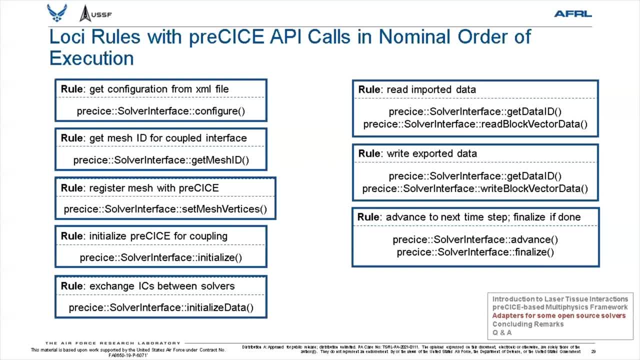 For the sake of time I won't go into detail on each of these rules, But there are different rules for registering the mesh And inside of that rule the associated API call to set the mesh vertices is called. There are rules for reading the imported data and writing the exported data. 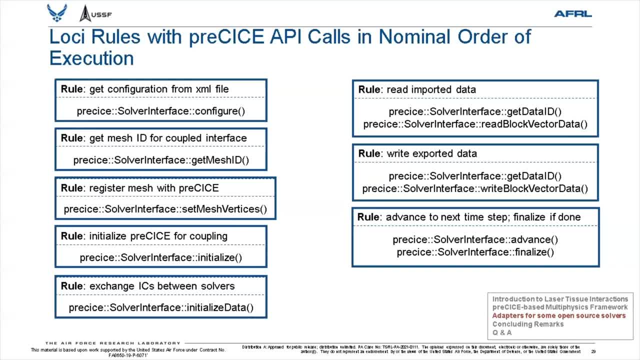 And the Precise API calls associated with those actions are contained in those rules, And there's also a rule to advance the solver to the next time step and to finalize an interaction with Precise when the simulation is finished. So the next rule is to get the configuration from the XML file. 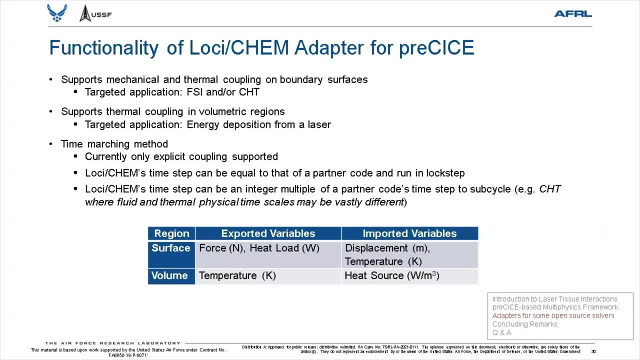 So we'll go into that in a second. So the next rule is to get the configuration from the XML file And, as you can see, the set up of this application is complete. The LociChem adapter supports mechanical and thermal coupling on boundary surfaces. 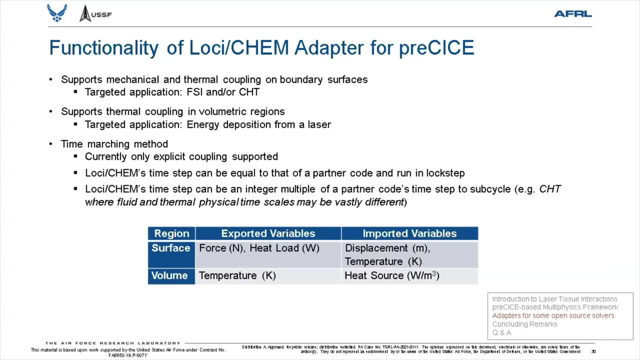 The targeted application here would be for fluid structure interaction and or conjugate heat transfer. It also supports thermal coupling in volumetric regions. This supports explicit coupling. LociChem's time step can be made equal to that of a partner code and they can run in lock step. 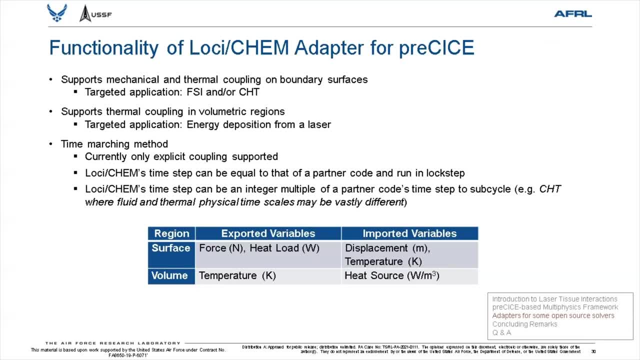 Or LociChem's time step can be an integer multiple of the partner code's time step, allowing it to sub-cycle. The use case here would be for conjugate heat transfer where, for example, the fluid and thermal physical time scales may be very different from one another. 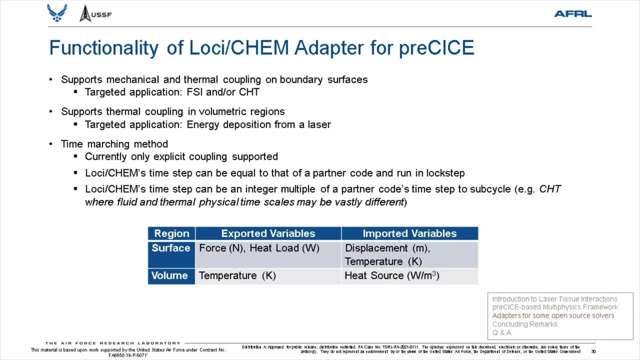 So you may not want to run the codes with the same time step. All of the data imported and exported in the adapter is done at the nodes For surface coupling. it's supported to export nodal force and nodal heat load and import a nodal displacement and nodal temperature. 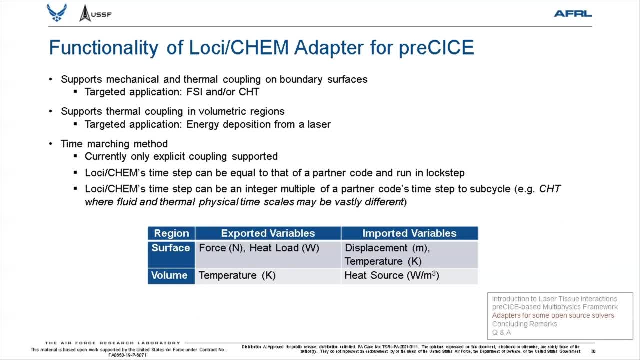 For volumetric coupling. it is supported to export a nodal temperature and import a volumetric heat source at the nodes. LociChem itself is a self-centered solver, So internally it needs data at face centers and cell centers. So the data it needs is interpolated from the nodal values that it receives from the adapter. 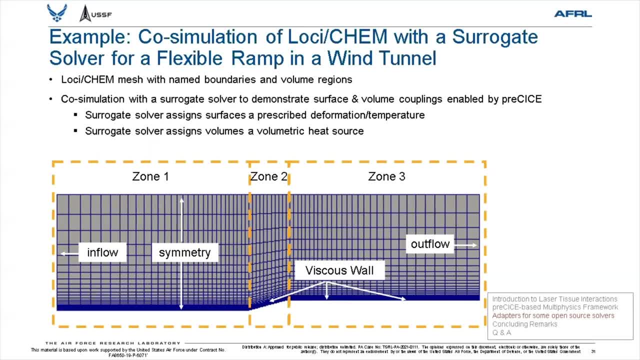 And I'll finish with an example. This is a co-simulation using LociChem and the PRECISE adapter with a surrogate solver for a flexible ramp in a wind tunnel. The purpose of this example is to just demonstrate that data is being exported. 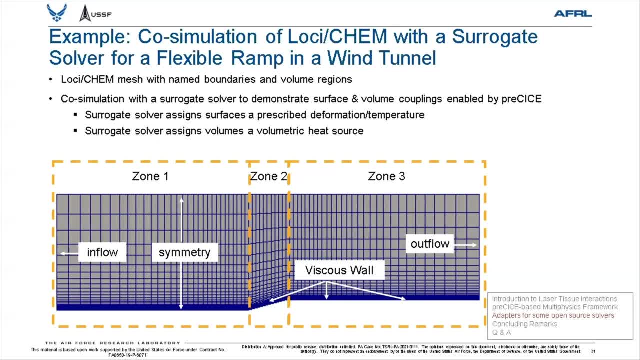 Data is being exchanged between the two solvers and the coupling is working as we expect it to. We're not trying to generate any specific flow results, So we begin with a LociChem mesh that has named boundaries and volume regions. There are three volume regions named Zone 1, 2, and 3, as shown in the schematic. 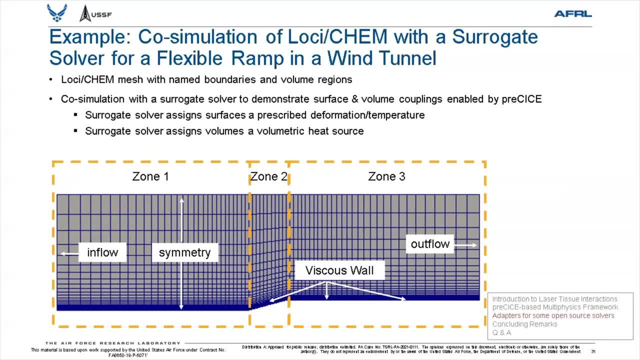 And there are named boundary conditions. We have an inflow boundary upstream and outflow boundary downstream. We have an inflow boundary upstream and outflow boundary downstream, And we have three distinct viscous wall boundary patches. The co-simulation with the surrogate solver is set up to exercise both the surface and volume couplings that are enabled by the adapter. 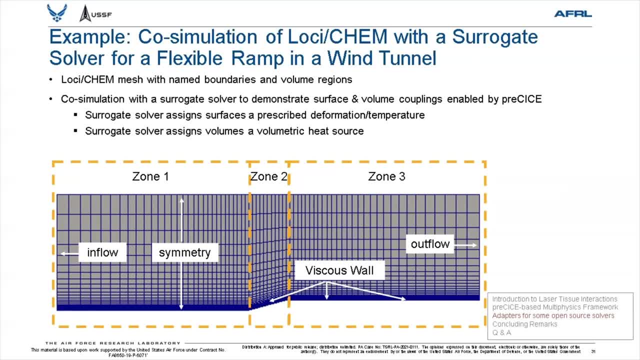 So for surface couplings the surrogate solver will pass a prescribed displacement for each of the three individual viscous wall boundary surfaces that are engaged in the coupling. The deformation will be sinusoidal over the individual patch. Thermal coupling is prescribed on just the ramp viscous wall boundary. 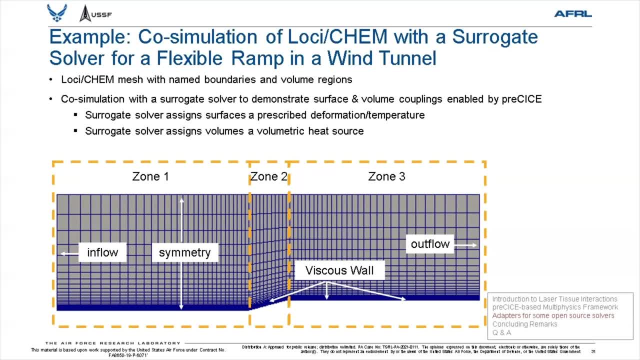 That's the upstream most boundary And again it's a sinusoidal prescribed distribution of temperature. Volumetric coupling is set up in Zone 3, where the surrogate solver will assign a volumetric coupling, The surrogate solver will assign a volumetric heat source. 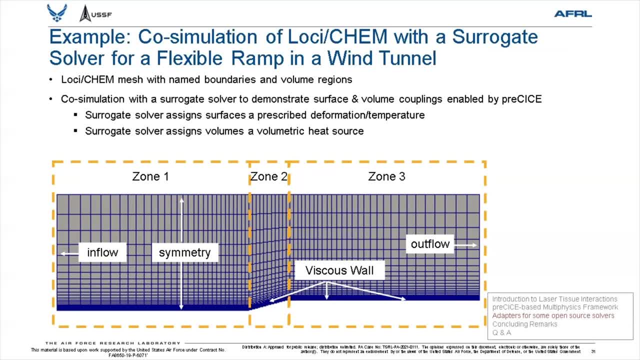 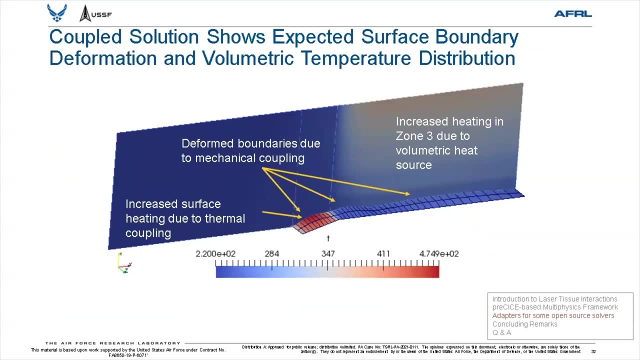 And this heat source will vary linearly and it will reach its maximum as we move away from the viscous wall. So here we see a contour plot of the coupled solution And it's showing the expected surface boundary deformation. You can see each of those three individual boundaries. 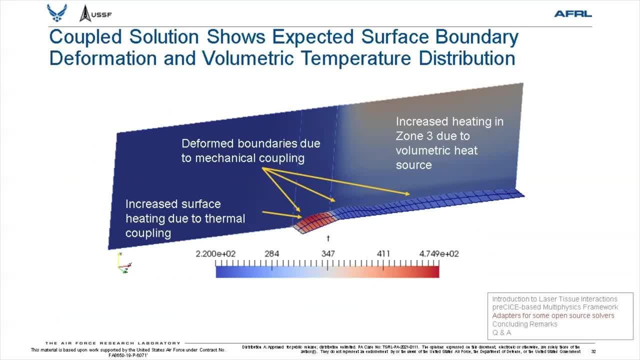 There's a hint of a sinusoidal deformation And that's a result of the surrogate code prescribing a sinusoidal deformation on each of those boundaries. On the ramp boundary, we see increased surface heating due to the sinusoidal temperature distribution that was prescribed by the surrogate code. 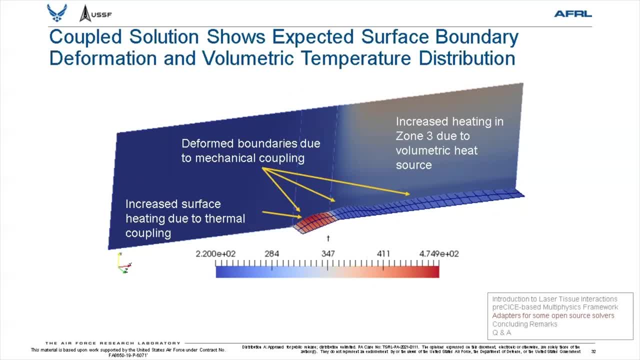 And then in Zone 3, we see increased heating due to the volumetric heat source that was prescribed, And that heating is larger as we move away from the viscous wall, As we move away from the wall, as expected. So this is showing that the precise adapter is allowing the exchange of surface and volume data and working as we expect it to. 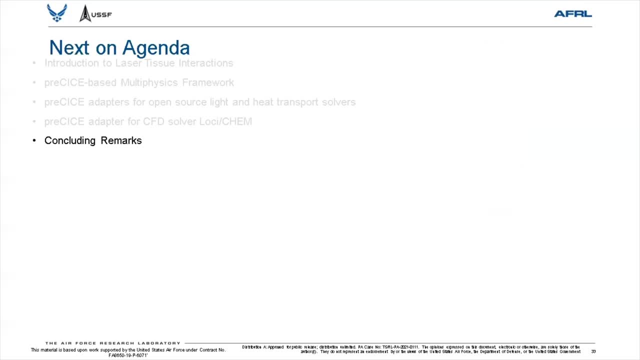 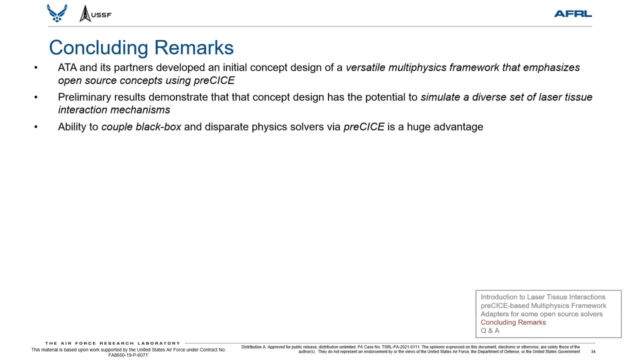 And now I'll pass it back to Satish for some concluding remarks. Thank you very much, Mike. So, on the whole, to conclude, I would like to say that we developed an initial concept, design and prototype of a precise-based, versatile multiphysics framework that's entirely open source. 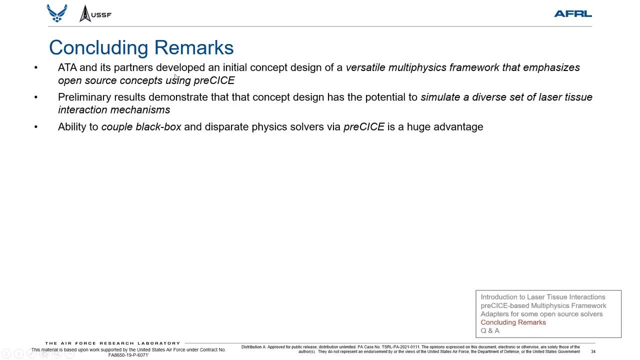 Second, by virtue of the working knowledge that we gained of the different components of the framework, and based on the preliminary results we generated, we think that this design has a huge potential to simulate many of the laser tissue interaction mechanisms that are of interest to us and to the community. 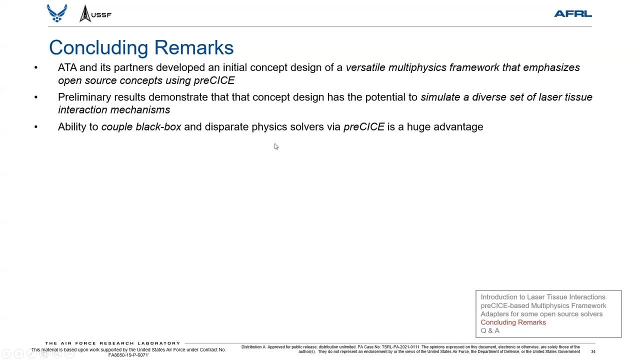 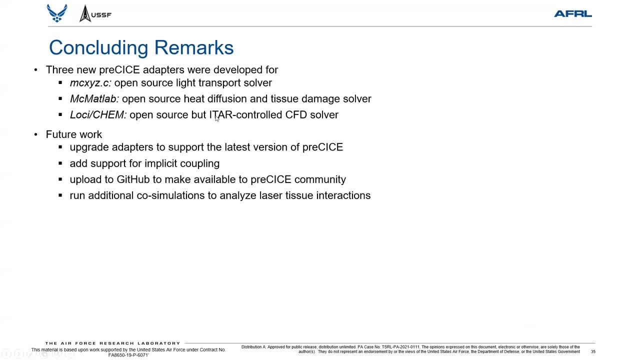 In general. the ability to couple black-box solvers and disparate physics solvers for precise is a huge advantage And we appreciate the Precise team for developing such a versatile and outstanding library. And just to be clear, we developed three new Precise adapters so far and all of them are for open source solvers. 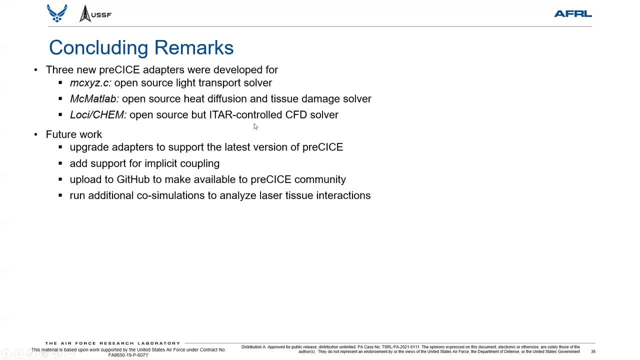 except LociCAM, which is open source, but I have control. As part of the future work, the plan is to upgrade adapters to support the latest version of Precise, add support for implicit couplings and make those available to the community via GitHub. 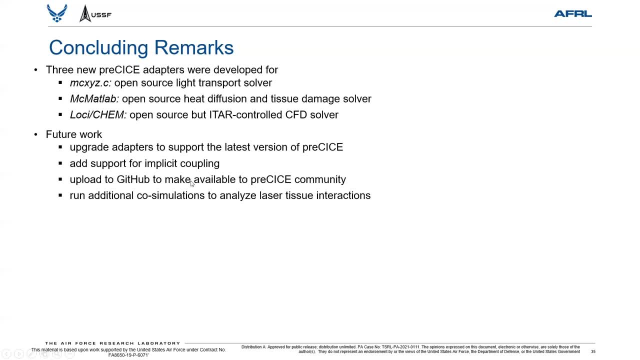 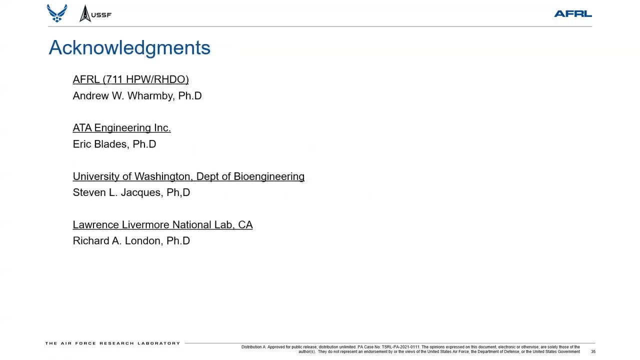 and then, most importantly, run additional co-simulations to analyze the many laser tissue interaction mechanisms of interest. I would like to once again acknowledge the financial support provided by the US Air Force and technical support provided by Dr Andrew Womby. I would also like to acknowledge the other project team members that include Dr Eric Blades of ATA. 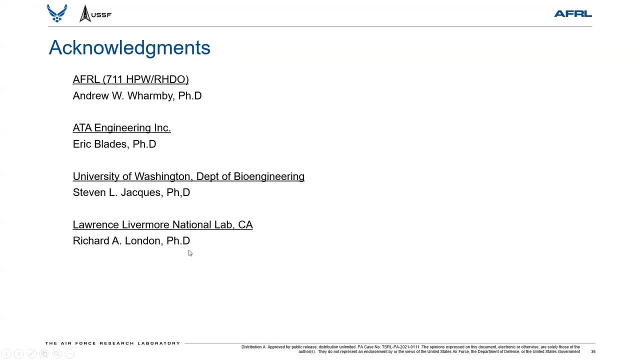 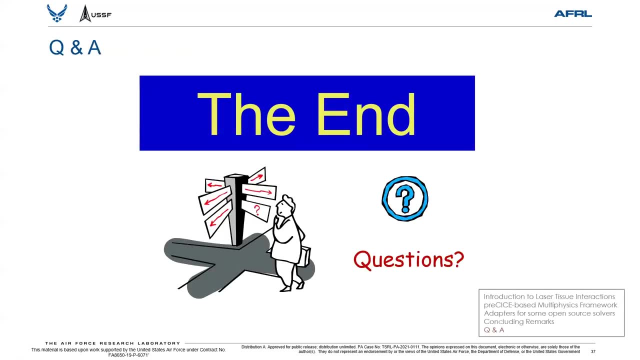 Professor Steven Jacks of the University of Washington and Dr Richard London of the Lawrence Livermore National Lab in California. That said, we thank you very much for your attention. We are now open to any questions you may have.